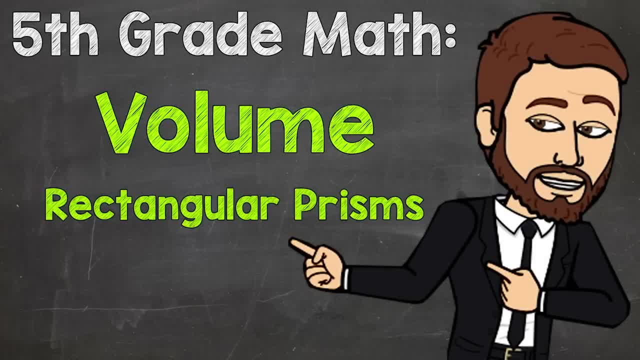 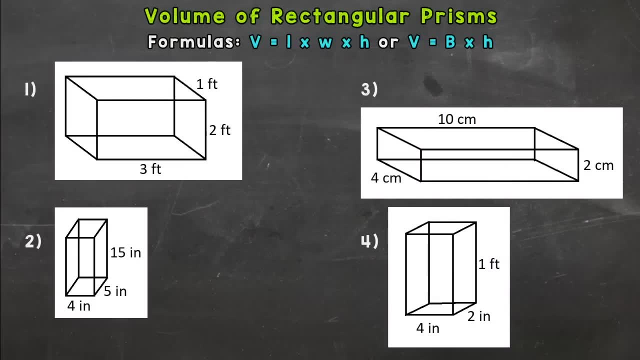 Welcome to 5th Grade Math with Mr J. So in this video we are going to be covering how to find the volume of rectangular prisms. Now, rectangular prisms are three-dimensional shapes, So what volume is is finding out the amount. 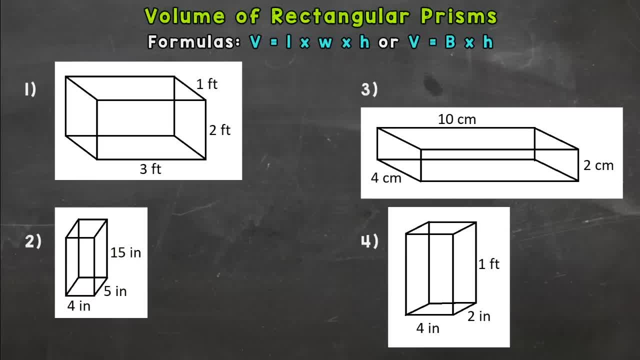 of space. that object takes up three-dimensional space. So there's a couple formulas we use- and they're up top here- to find the volume of a rectangular prism. Now we're going to hop in the number one and just go through a few examples here so you can get this down Now. the V stands for volume. in our 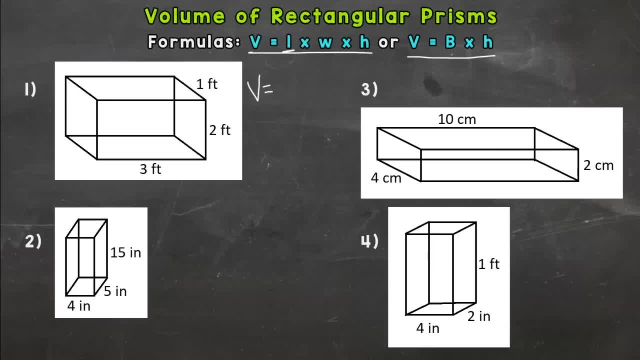 formula. and then this L right here stands for length times width, times height. or another formula you may see is this capital B, which stands for revised volume, the area of the base times the height. Now, these formulas are basically the same thing, because length times width will give you the area of the base, the area of the base which you just 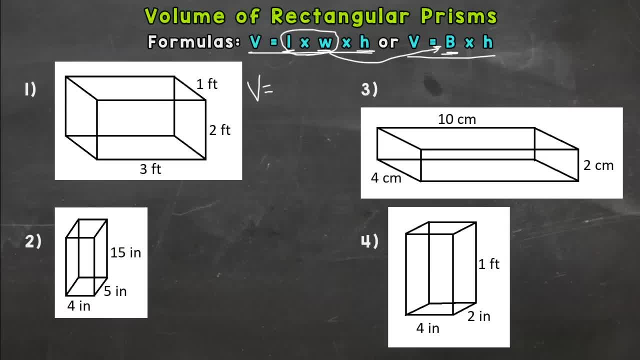 multiply by height. So either way, you're going to get the same answer and they're basically the same thing. I'm going to use this one right here: length times, width times, height. So I always like to write my formula out. this is always a good habit to get into, and then we're going to plug in. 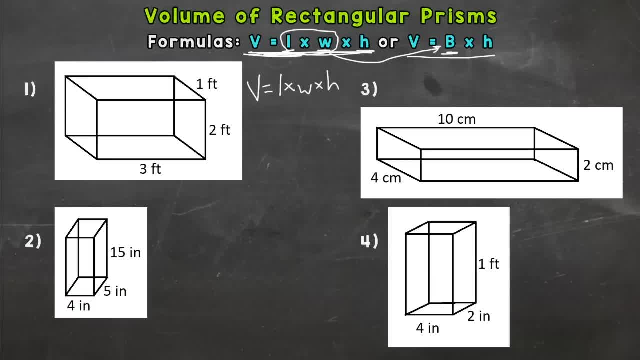 our values for length, width and height. So volume equals length times width times height. Now we go over to our model here and we see the length is one foot times our width right here is three feet times our height, which is two, Two feet. Then we multiply those together and that will give you the volume of that rectangular. 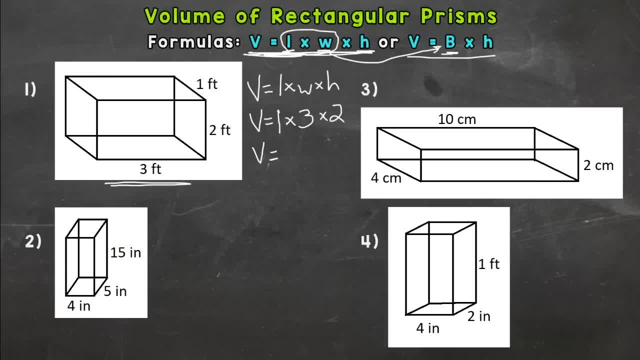 prism. How many cubic feet would fill that prism, How much space it takes up. So one times three is three, times two is six. Now we always want to label our answer and we look back at our model and we see feet and what we do for volume is we put a little three up here and this means 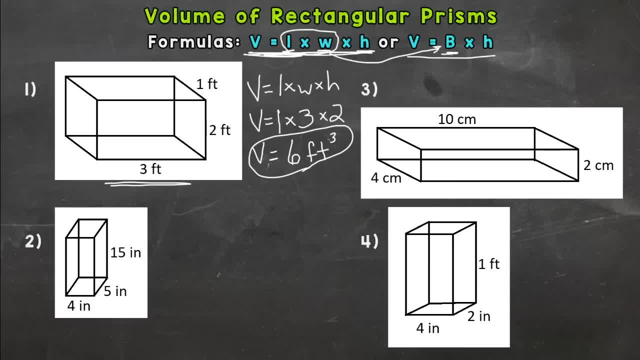 six cubic feet. Okay, six cubic feet, That's how many cubic feet it would take to fill that rectangular prism. Or you could say six feet cubed either one. Now let's go to number two here. Write out our formula: volume equals length times width, times height. Plug in length. going back is: 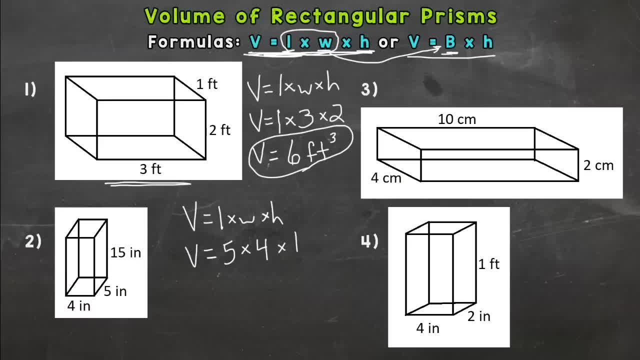 five. Our width is four and our height is five, So that's 15.. So what we would do now is multiply these out and we would get to 300 inches cubed or 300 cubic inches. Five times four is 20, times 15 is 300.. 300 inches cubed. 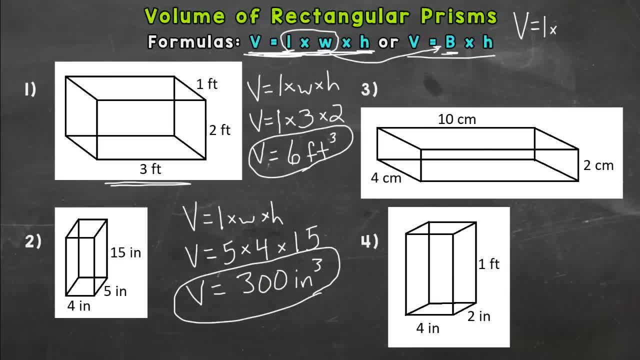 All right, let's go to number two. here We would get to 300 inches cubed. Number three: volume equals length times width times height. Plug in our length going back is four. Our width is 10 and our height is two centimeters. So we multiply out four times 10 is 40 times 280 centimeters cubed. 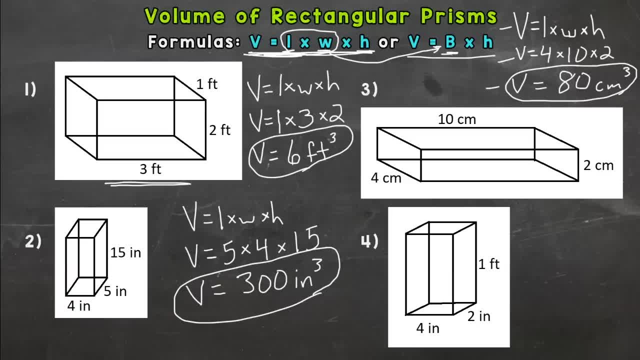 Formula plug-in answer. And then let's go to number four. Now there's something special about number four, and I put this in very specifically because you have to pay attention before you start some of these problems. One thing should pop out about the height on this rectangular prism: It doesn't make 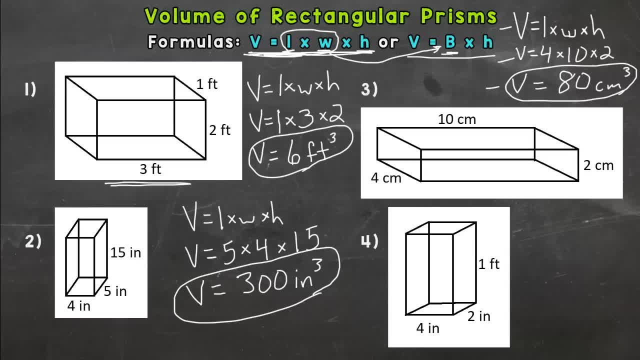 sense in comparison to the others. As you notice, the width is four. That side is not as long as that one foot. It's because we have inches here and this is feet for our height. If that happens, you need to convert everything to the same unit of measurement. It's going to be easier to convert. 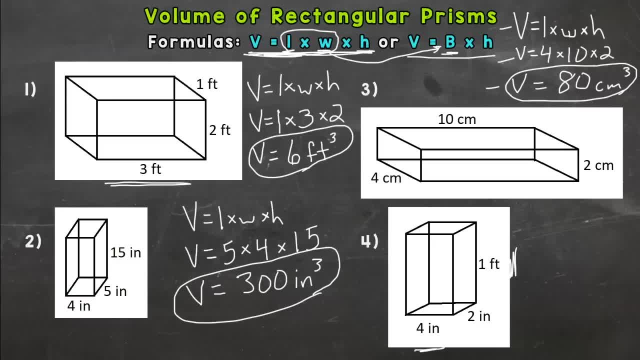 feet into inches and then plug in. So one foot is 12 inches. So we know our height is going to be 12 inches. Now everything's in inches and we're good to go. So formula: volume equals length, length Times, width, times height. Plug in: Our length is two inches, Width is four And our height is 12. 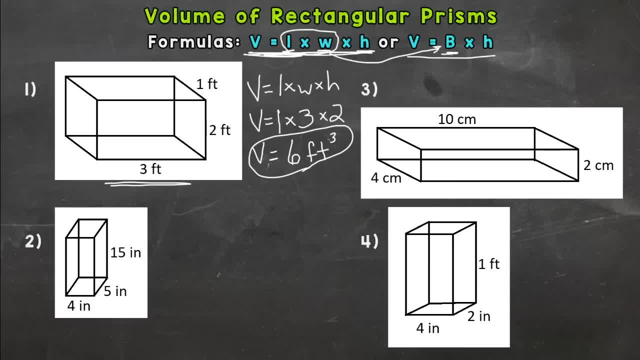 six cubic feet. Okay, six cubic feet, that's how many cubic feet it would take to fill that rectangular prism. Or you could say six feet cubed either one. Now let's go to number two here. Write out our formula: volume equals length times width, times height. Plug in length. going back is: 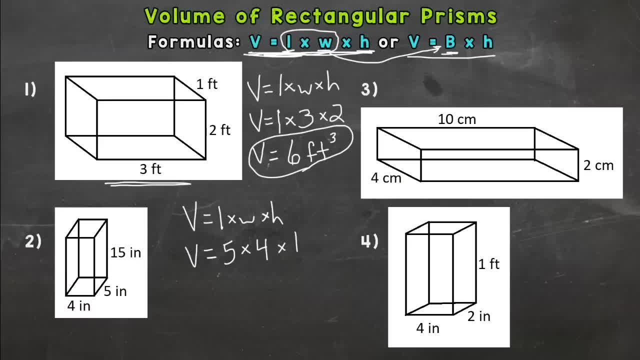 five. our width is four and our height is five, So that's 15.. So what we would do now is multiply these out and we would get to 300 inches cubed or 300 cubic inches. Five times four is 20, times 15 is 300.. 300 inches cubed. 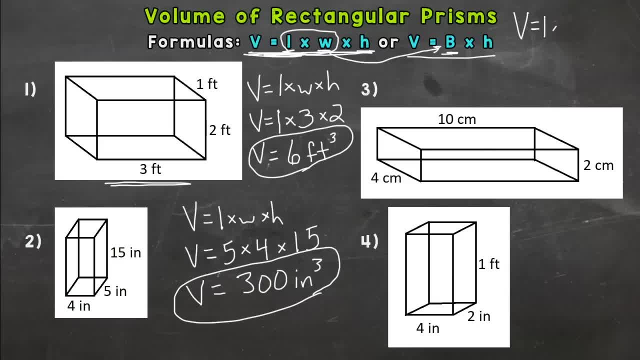 All right, let's go to number two. here We would get to 300 inches cubed. Number three: volume equals length times width times height. Plug in: our length going back is four, our width is 10 and our height is two centimeters. So we multiply out four times 10 is 40 times two. 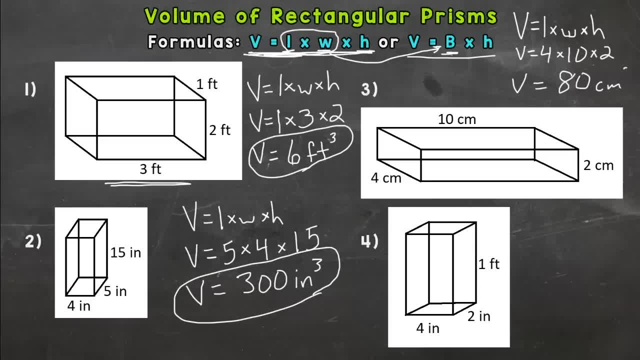 80 centimeters cubed. So we multiply out four times 10 is 40 times two: 80 centimeters cubed. Formula plug in answer. And then let's go to number four. Now there's something special about number four, and I put this in very specifically because you have to pay attention before you. 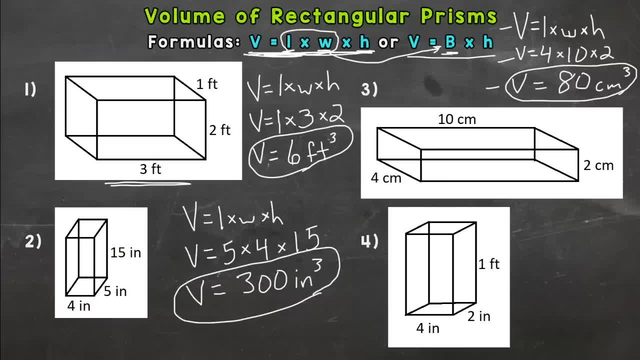 start some of these problems. One thing should pop out about the height on this rectangular prism. It doesn't make sense in comparison to the others. As you notice, the width is four. That side is not as long as the other side, So we're going to put in four, And then we're going to put in four. 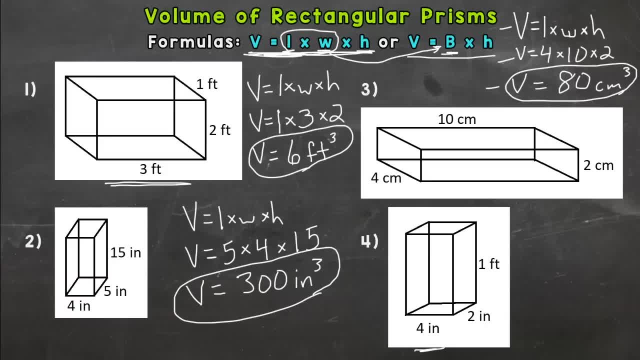 Kind of like cutting off a big sheet. Ever since healingzy did that, everything is now the same. That's 차 comparatively wonderful. One of the things we need to be interested in tagging along is that one foot- it's because we have inches here and this is feet for our height. 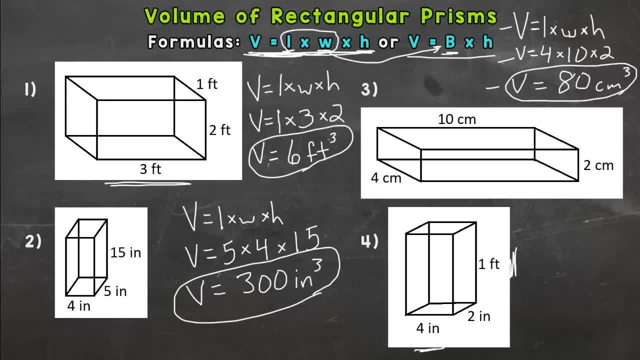 If that happens, you need to convert everything to the same. если unoEV unit of measurement, It's going to be easier to convert feet into inches- not even feet- and then plug in. So one foot is 12 inches, So we know our height is going to be 12 inches.